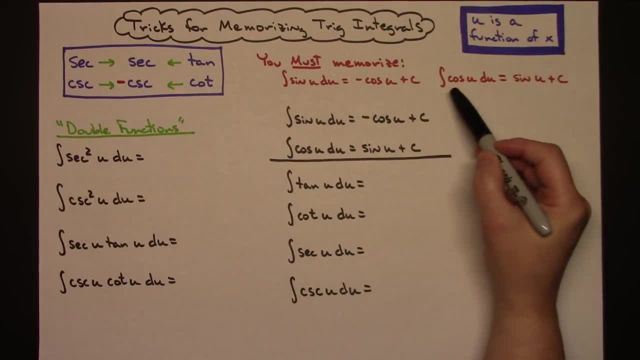 as being negative cosine u plus c And your integral of cosine u du is sine u plus c. Alright, those two things. If you've got the derivatives memorized. since you know derivatives and integrals are inverse functions, it should be easy for you to memorize those two. 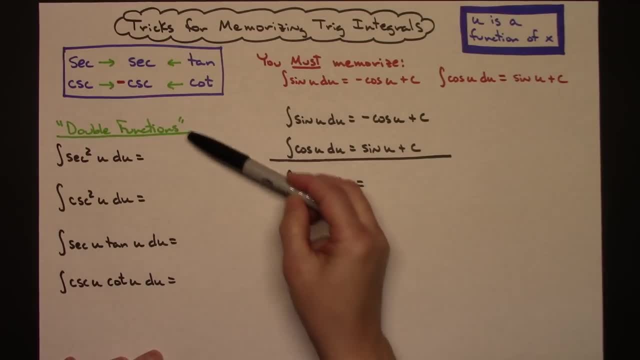 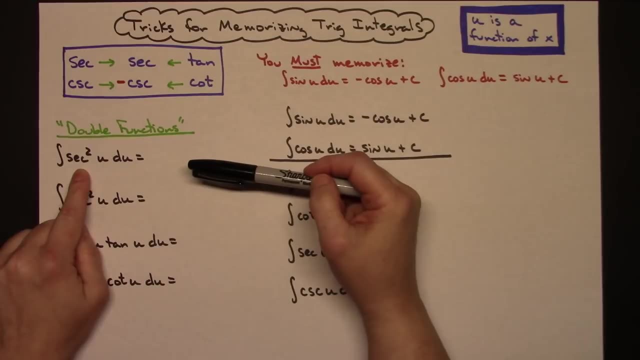 Alright, I think, to walk you through this to begin with, I think I want to start over here with these What I call double functions. Alright, I call them double functions just because I've got secant squared, so it's secant, secant. 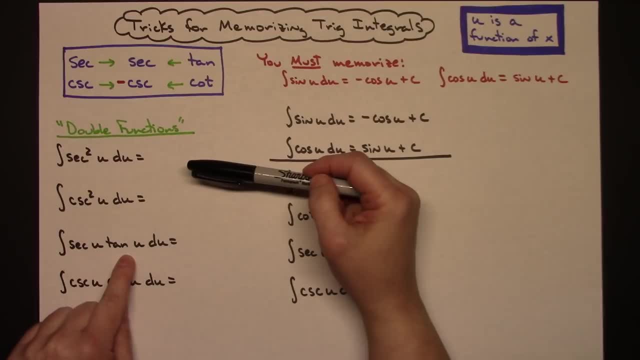 It's like two functions. Down here I've got like secant tangent, so I've got two functions, Alright, so each one of these have two functions in them, so, referring to them as double functions, All four of these will come straight from this chart. 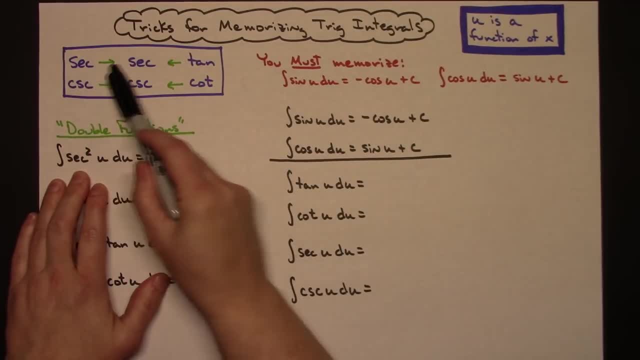 Okay, so if I want to integrate secant squared u, alright. I can look at my top row. right there I've got secant squared, so I've got secant secant. The only thing left on that row is a tangent. so then that means the integral is tangent u plus c. 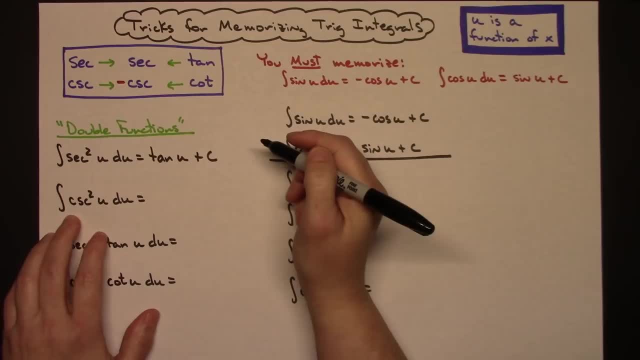 Straight from the chart. Alright on this one. I've got the integral of cosecant. squared u, Alright. so I'm going to come up here to the bottom row. I've got two cosecants, so there's cosecant, there's cosecant. 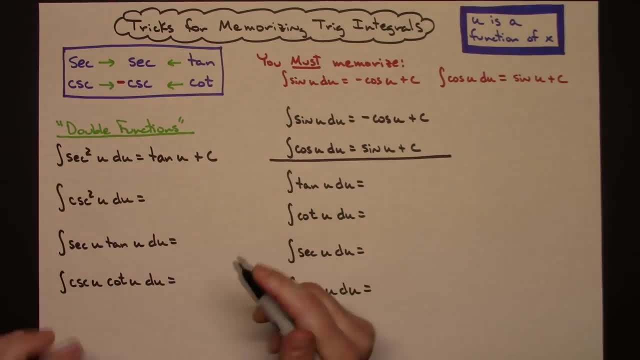 so the only thing left on that row would be negative cotangent. Alright, so my integral is negative cotangent u plus c. Alright, for the third one. here I'm integrating secant tangent. Alright, again, I'm going to come up here to my chart. 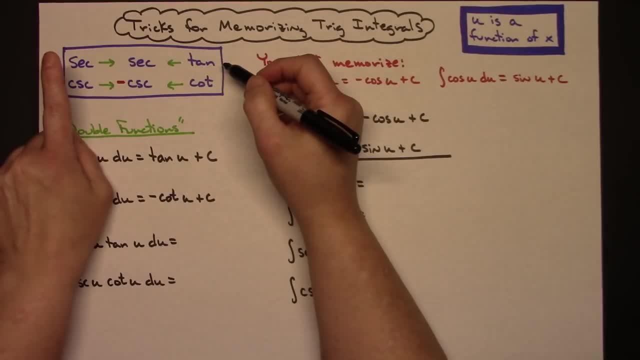 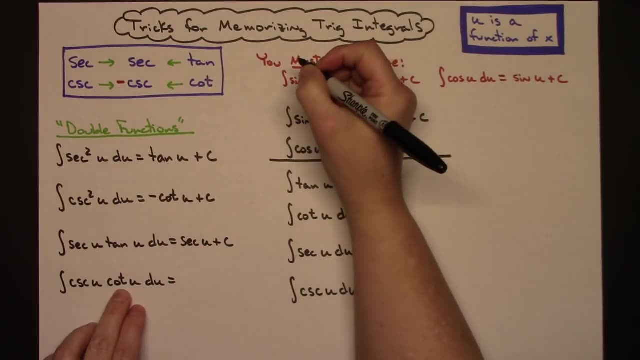 I've got secant and tangent right there. The only thing left over there then would be the secant. So this is secant u plus c And cosecant cotangent. looking at this bottom row right here, I've got a cotangent and cosecant out here. 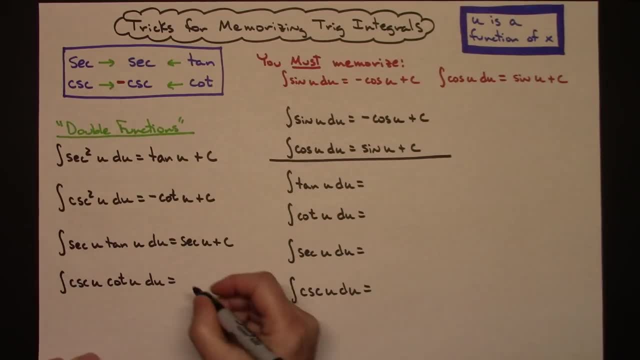 The only thing left then would be that negative cosecant there in the middle, So the integral. there would be a negative cosecant u plus c. Alright, so those four are pretty easy to remember. If you remember they're all the double angles. 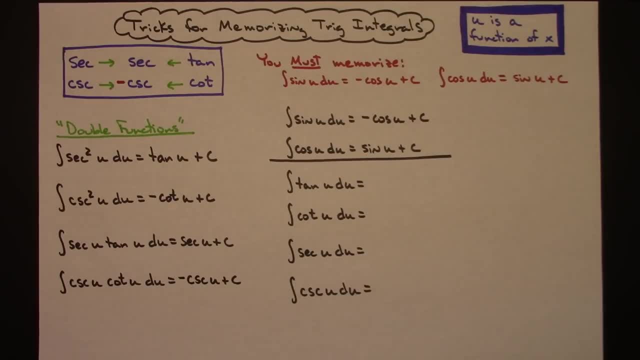 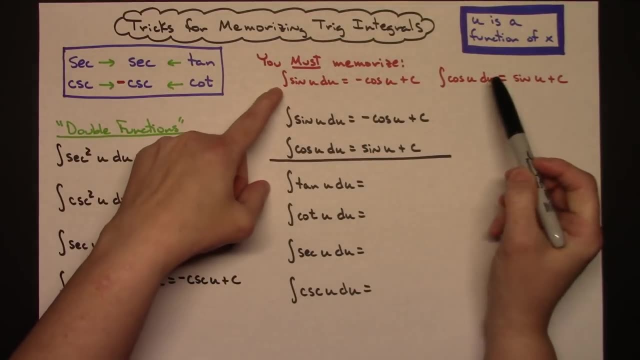 and they come right from that chart. Okay, now for all of the single trig integrals, the sine and cosine I went ahead and wrote down because you've already got those memorized. So if you start with those two, then these other four are right here in the chart. 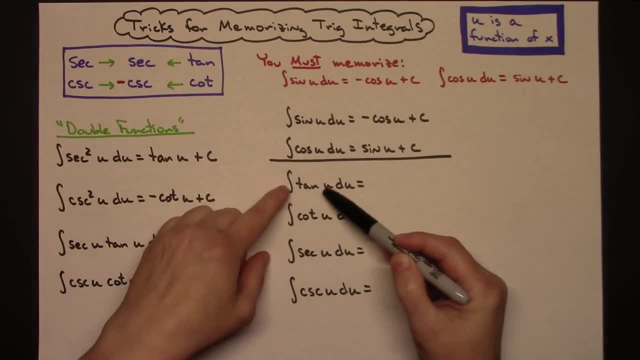 Tangent, cotangent, secant and cosecant. Alright, now, the reason I chose to do these two and then these two last is because these two right here are. you're going to use your sine and cosine to help you come up with those. 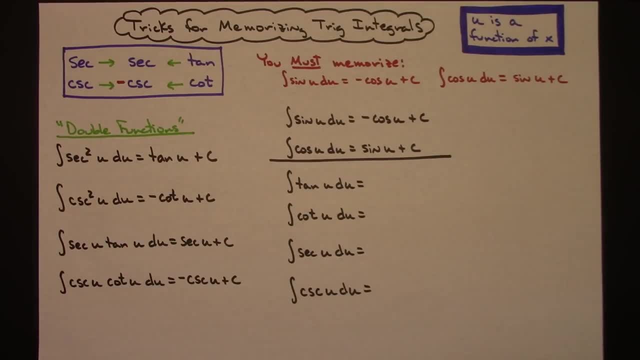 Alright. now I did draw a little line here. These four are going to be in our log functions, So every one of these integrals will have natural log, Alright. and then every one of the natural log ones also have the absolute value bars. 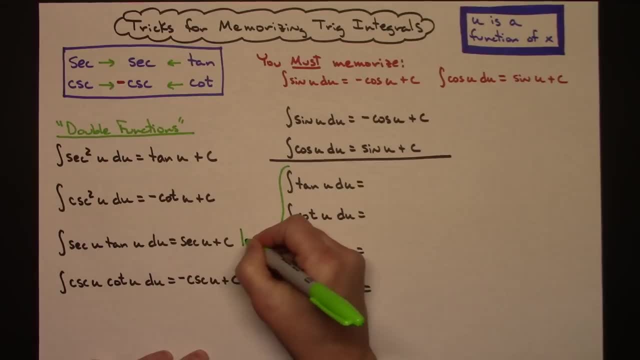 So that's kind of why I separated it from these first two right here. So natural log and absolute value bars. Okay, Alright. So now I said you're going to use these two answers right here to help with these two, because this chart doesn't work. 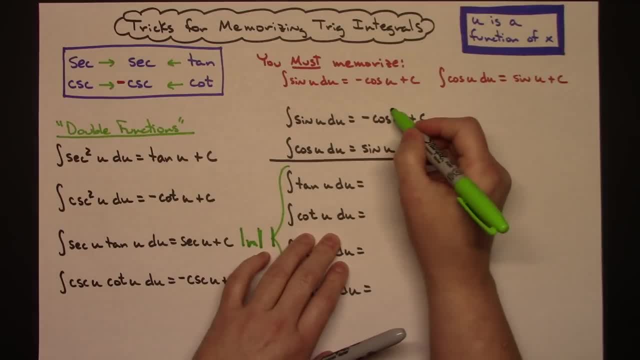 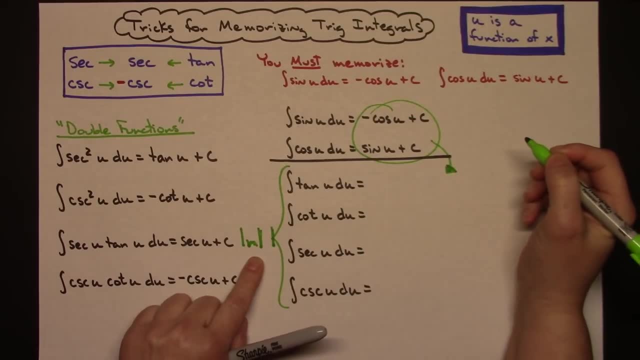 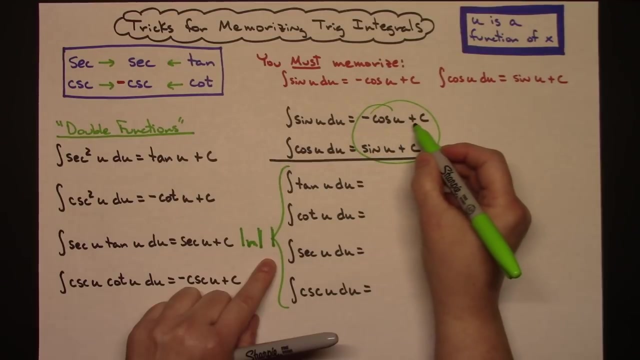 Alright, so literally, what you're going to do is you're going to take the answers there and just bring them down. The only thing you've got to add is your natural log and your absolute values. Okay, so, since this top one right here is minus cosine u plus c. 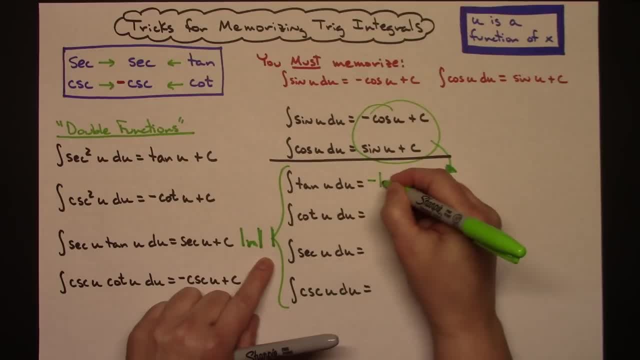 I'm going to have negative, I'll pull it out in front. natural log, absolute value, cosine u plus c. Alright, and then same thing here. I'm going to bring this one exactly straight down here, but I'm going to add natural log and absolute value to it. 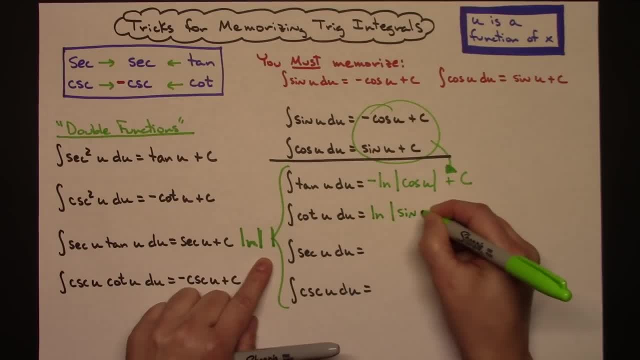 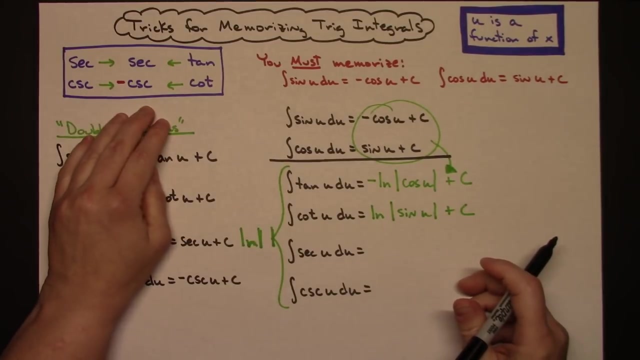 So I'll have natural log: absolute value sine u plus c. Alright, so these two do not come from this chart. They come from the two that you have memorized up there on sine and cosine. all right, now these bottom two are going to come back from here. all right, and 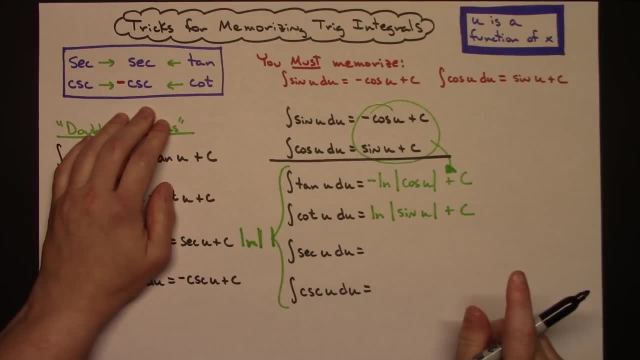 there is one extra thing that if you did watch my video on the trig derivatives, I'd made a comment that only in that one, where double functions and derivatives are multiplied as answers, okay, well, here we are going to have some double functions as our answers, and in integrals. then you've got to remember.